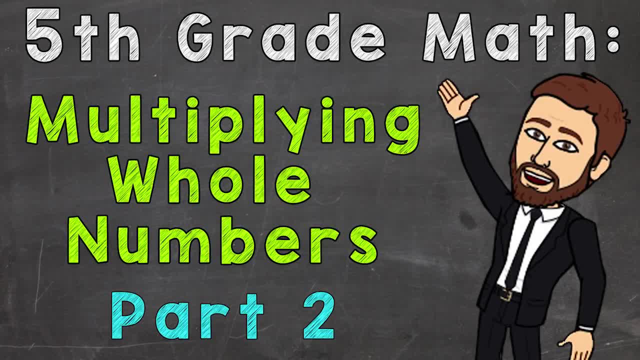 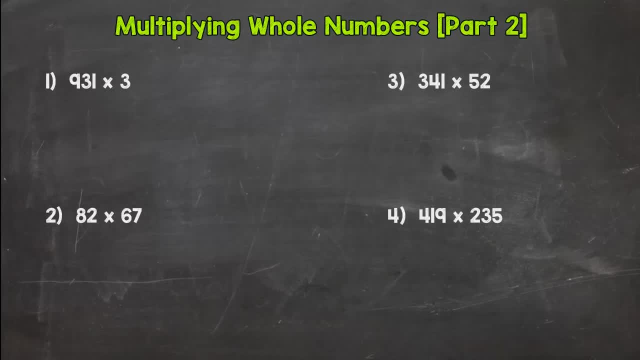 Welcome to 5th Grade Math with Mr J. So here we are at Multiplying Whole Numbers, Part 2.. If you missed Part 1, I put the link in the description. So check Part 1 out and then you can come back to Part 2.. 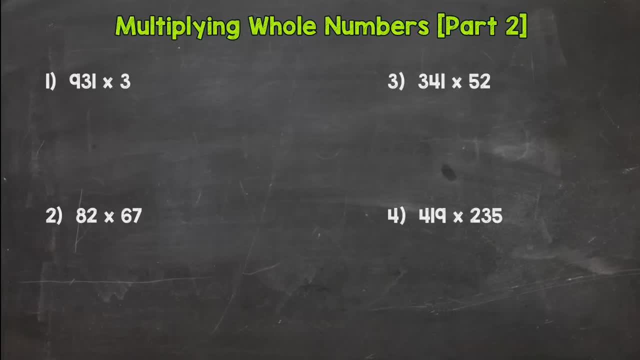 So these are instructional videos on Multiplying Whole Numbers, And after we get through Part 2, you can hop over to the Mastery Check where you can test your skills to see if you have it down. So much like Part 1,. we have four multiplication problems. 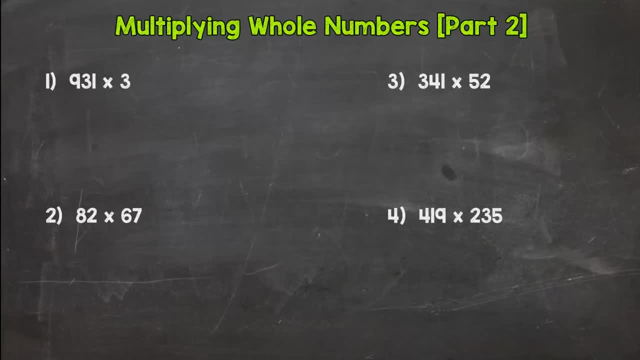 we are going to go through together And then, like I said, you will do the Mastery Check on your own to see if you have it down. So you should have a piece of paper and something to write with, because you will go through these problems with me. 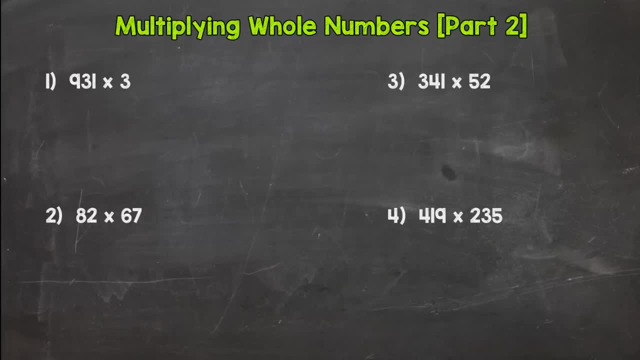 That will be much more beneficial than just sitting there listening to me talk. So we're going to start with number 1 here And we have a 3x1,, a 3-digit number by 1 digit, And as we go through we will increase in difficulty. 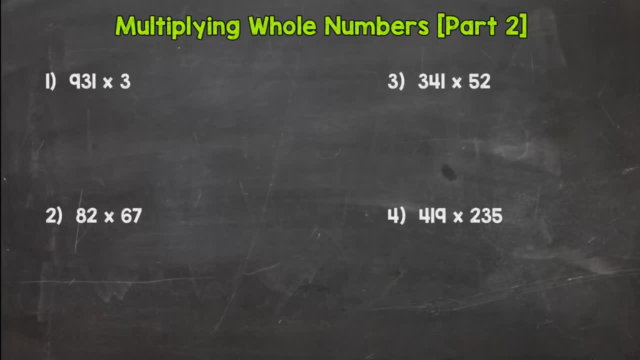 Like number 2, we have a 2x2.. Number 3, a 3x2.. And then number 4, a 3x3.. Alright, so we're going to rewrite these problems vertically, which means up and down. 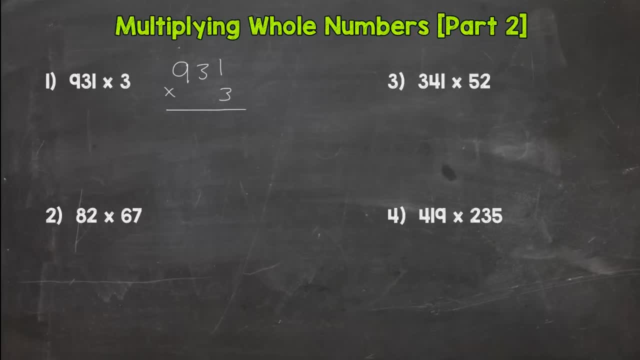 And then just go through our multiplying, our multiplication process here. So we take the 3 to the 1. 3 times 1 is 3.. 3 to the 3. 3 times 3 is 9.. And 3 times 7, 27.. 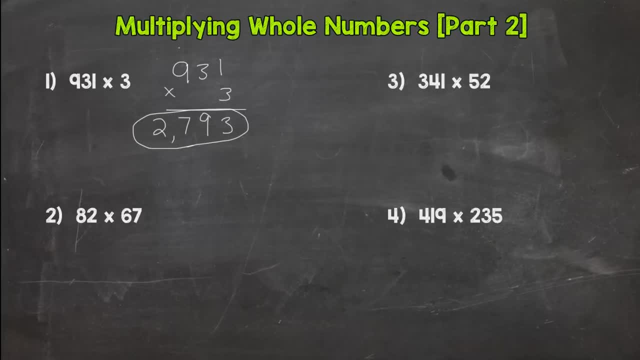 Put our comma in, We are done 2,793.. So, like I mentioned in Part 1, knowing your multiplication facts is very, very important here, because all this is is just repeated multiplication facts, making sure you have stuff lined up. 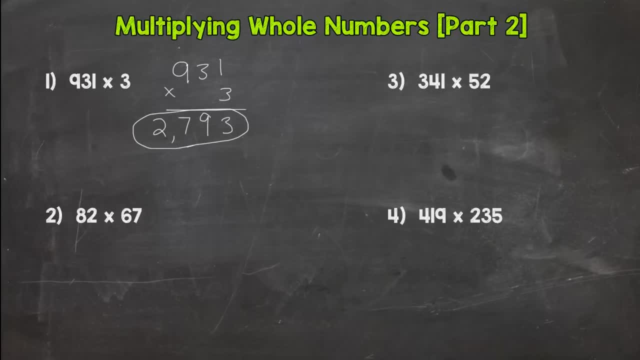 remembering placeholder zeros. and yeah, that's about it. So if you know your facts, very helpful here. So let's go to number 2.. We have a 2x2.. So in this one we are going to have two partial products that we add together. 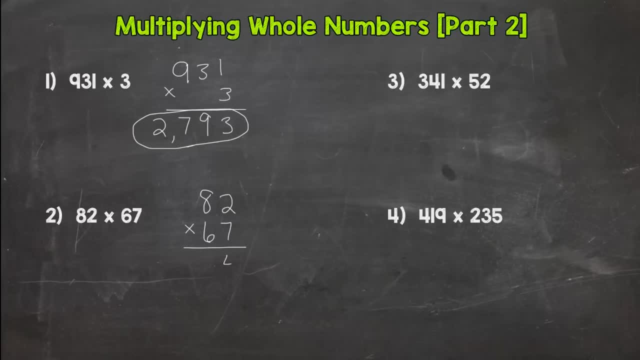 Remember we don't go: 7 times 2 is 14, and then 6 times 8 is 48, plus 1 is 49, and circle our answer Alright Incorrect. Okay, You have to take the 7 to the 2 and the 8,. 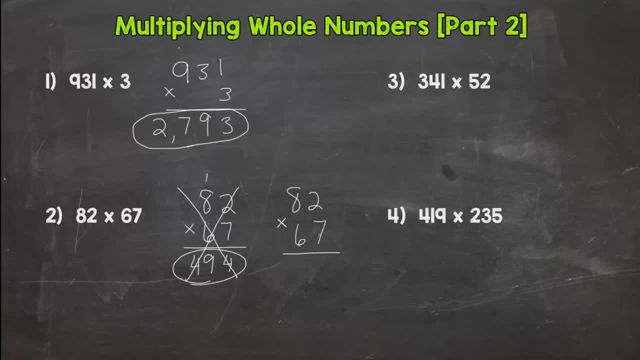 and then the 6 to the 2 and the 8.. So let's start with: 7 times 2 is 14, and then you take the 7 to the 8.. 7 times 8 is 56, plus 1 is 57.. 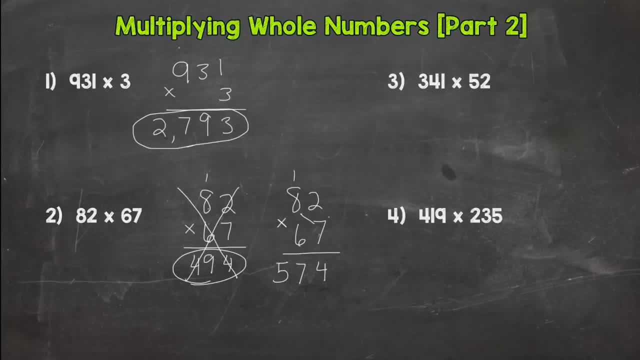 So would that be our answer? Are we done? No, We're done with the 7,. so we can cross that out and we're done with this regrouped 1.. So we can cross that out, So we don't get confused later if we have any other numbers up top there. 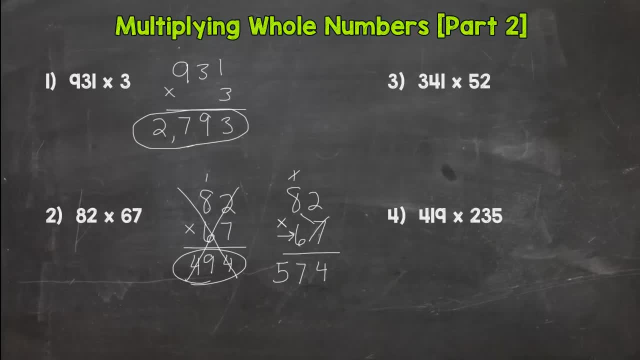 So the value of this 6 right here is 60. So we put a placeholder 0 here to make that 6 worth that 60. So and then we start with: 6 times 2 is 12, and then 6 times 8 is 48, plus 1 is 49.. 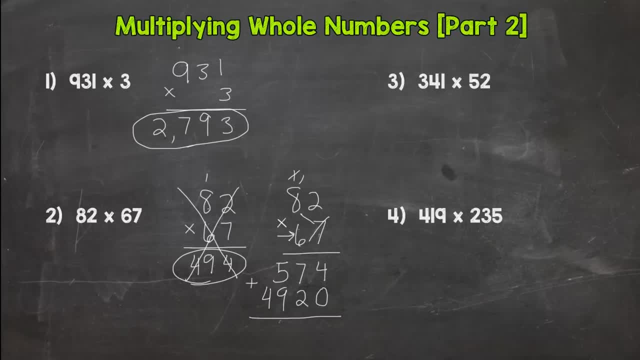 Now we're ready to add our partial products. These are our partial products. We add them together to get our product, which means answer to a multiplication problem. So 4 plus 0 is 4,, 7 plus 2 is 9,, 5 plus 9 is 14,. 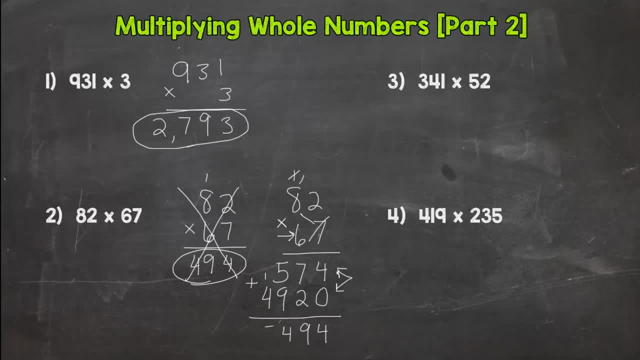 and then 1 plus 4 is 5.. So 5,494.. All right, let's step it up a notch. here We have a 3 by 2.. Same rules apply, So 5,494.. Take the 2 to every number and then the 5.. 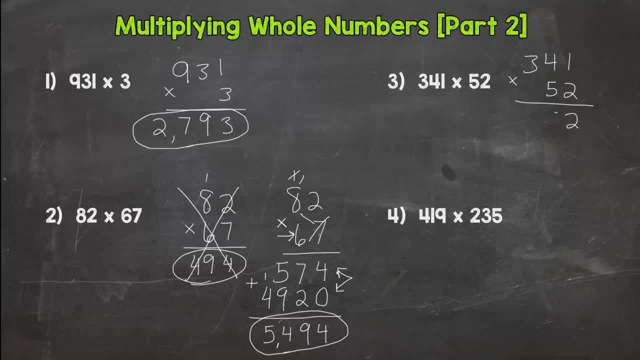 So 2 times 1 is 2,, 2 times 4 is 8,, 2 times 3 is 6.. Done with the 2.. All right, now we need to take that 5,, which has a value of 50.. 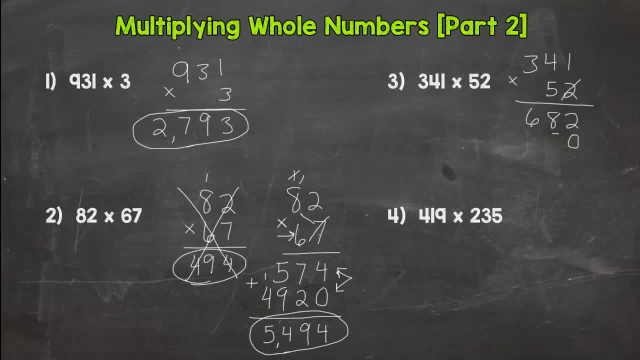 So we need a placeholder: 0.. 5 times 1 is 5.. 5 times this, 4- right here- is 20.. And then 5 times 3 is 15, plus 2 is 17.. See how we have to be nice and lined up here for our last step, when we add: 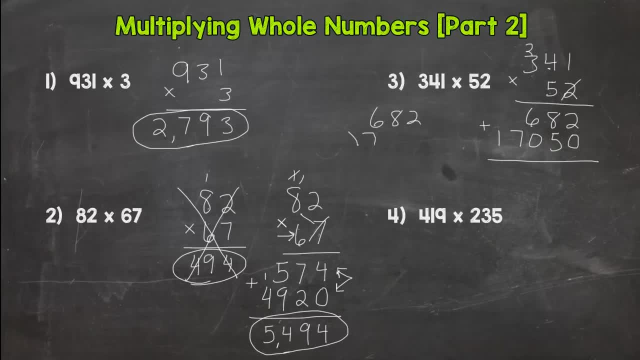 Take a look over here to the left. Let's say, if you have all of your numbers like this and you need to add them up, there's no way of knowing. okay, 2 plus 0 is 2, and then the 5 to the 8,. 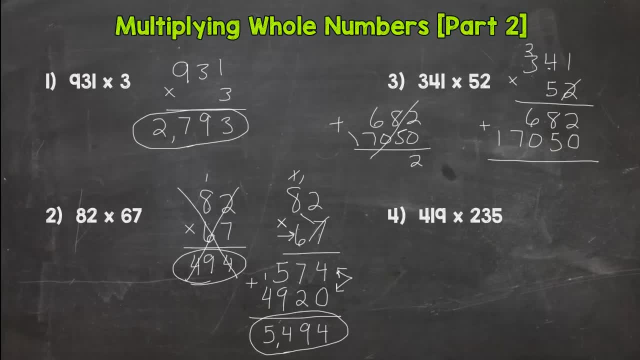 or is the 8 to the 0? You know. so make sure you are nice and neat and everything is lined up. 2 plus 0 is 2,, 8 plus 5 is 13,. 1 plus 6 is 7,, 7,, 1.. 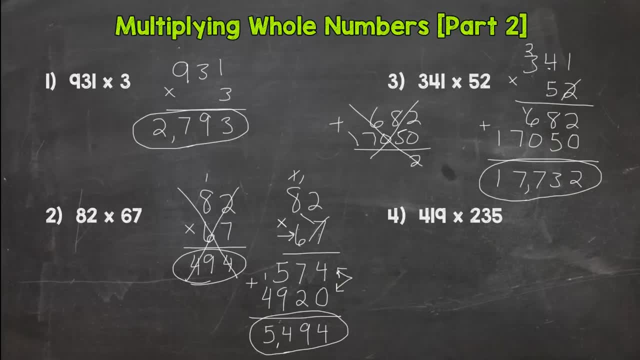 17,732.. And then, lastly, we have a 3 by 3.. A little extra step here, But nothing really that different. So let's take the 5 to each digit. 5 times 9 is 45.. 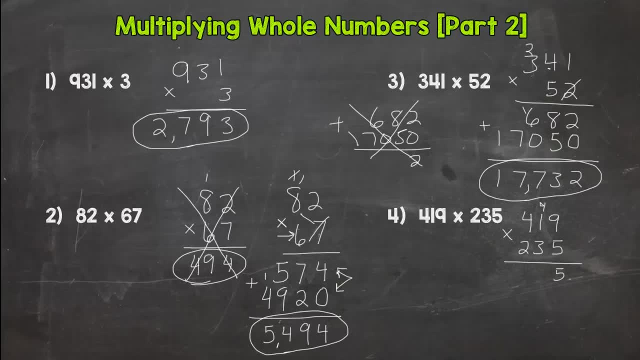 5 times 1 is 5, plus 4 is 9.. 5 times 4 is 20.. Done with the 5,, done with the 4. This 3 right here is worth 30, so let's put our 0.. 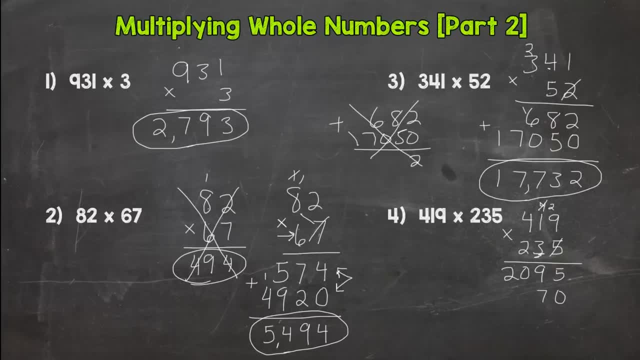 3 times 9 is 27.. 3 times 1 is 3, plus 2 is 5.. And then 3 times 4 is 12.. Done, done. Now our next step. don't forget, we have this 2 here. 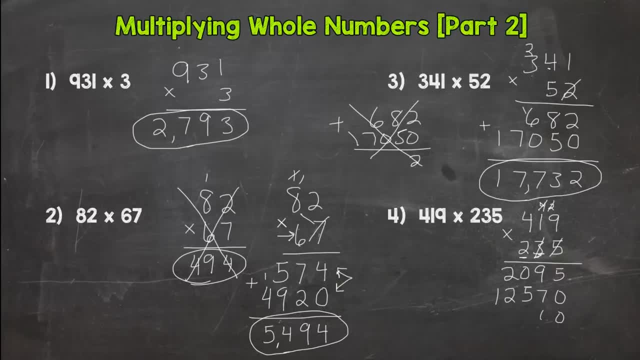 And that 2's value is 200, so we need 2 placeholder 0s. 2 times 9 is 18.. 2 times 1 is 2, plus this 1 up here is 3.. And then 2 times 4 is 8..